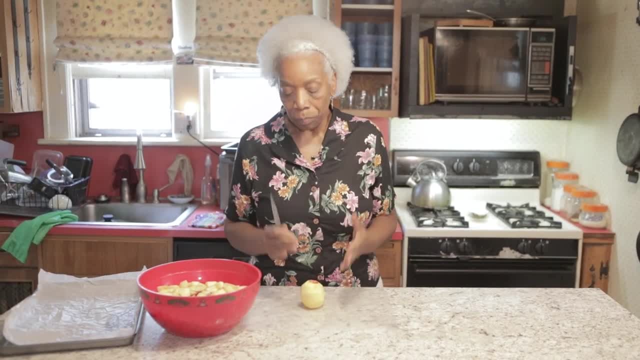 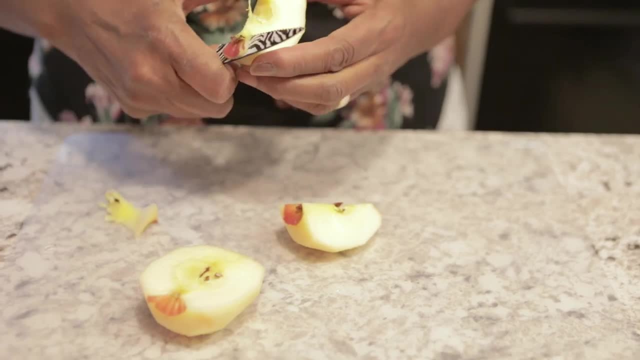 to do it. I have an apple in here that's soaking. You peel them, you cut them however you really like it. You cut it for pies, cakes, muffins And what you soak it in. How it soaks is: you take a. 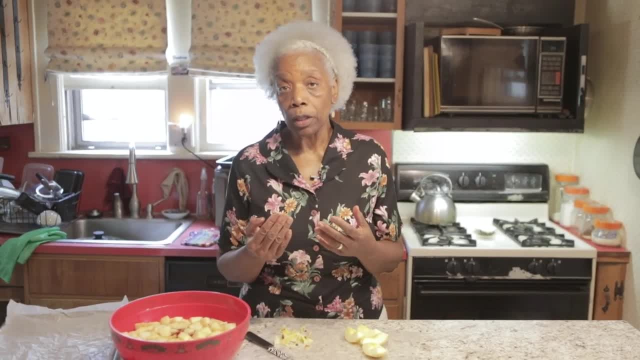 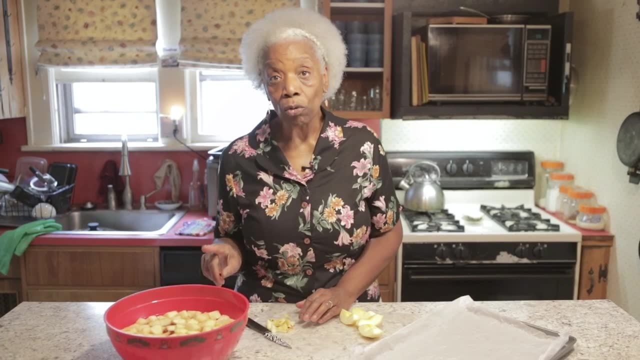 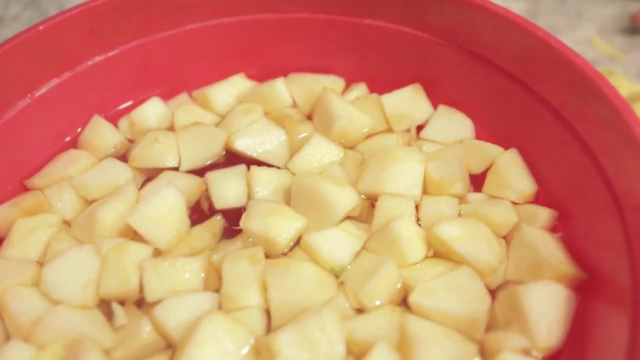 gallon of water. For every gallon of water that you have to soak your apples, use a tablespoon of lemon juice. You put the apples in the lemon juice so they don't oxidize. They stay as as white as they normally are. These are a little bit, but not much, because apples float, So what? 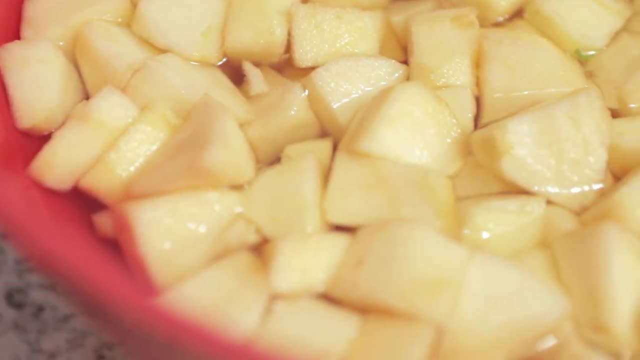 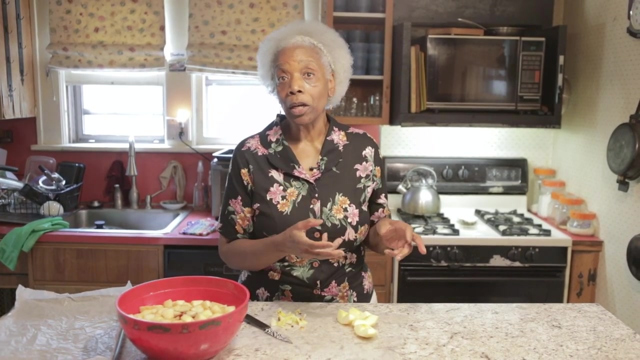 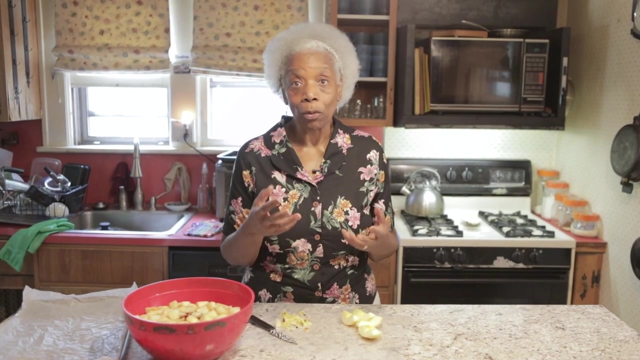 was exposed to the to the light got a little bit brown, but not very much. I only had six apples. I got them on on on a bargain markdown with old, old fruits and vegetables in my grocery store And they were all- mostly all organic. So I thought I'm going to get these And I wanted 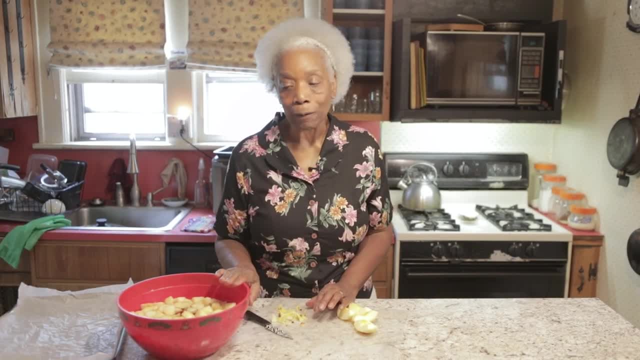 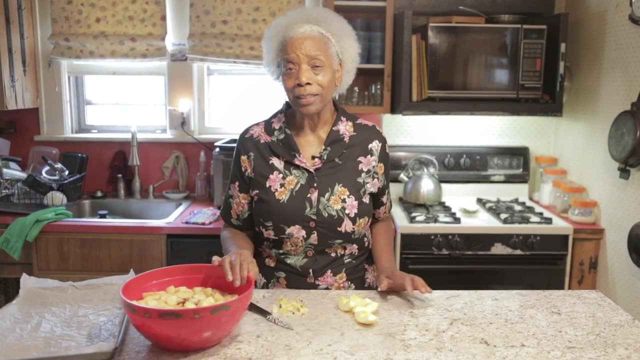 to freeze them, But I wanted to show you how to do it too, Because it's really easy. Now, why I do apples is not only for pies and stuff like that, but also because, for me, I like bananas, but the nice cream that I have, which is another video. 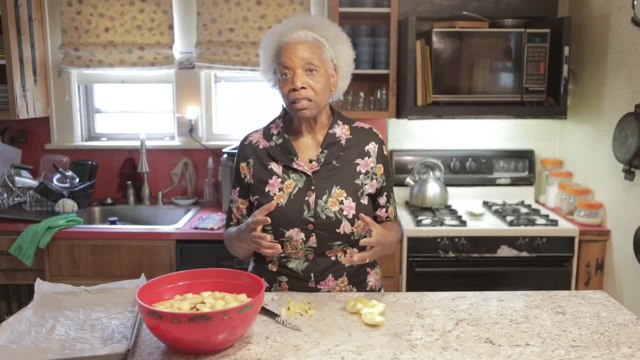 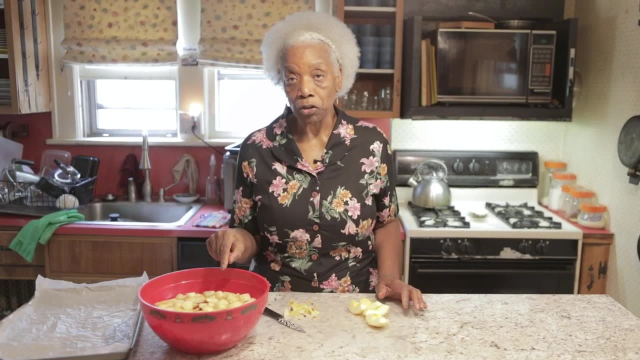 it. I'm not real crazy about bananas, And so what I do is I take a handful of small handful of frozen apples, fresh apples, and I throw it in the nice cream with the, with the banana, And it really calms the, the taste of the banana down. 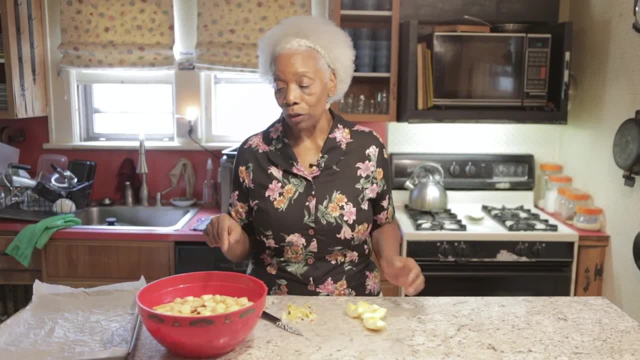 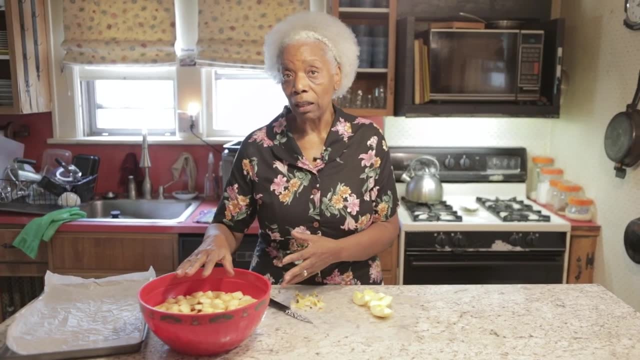 I don't know if that's something you want to do, but that's how it all started with these learning about frozen, frozen fruits and veggies. So this is about. this is a half a gallon. I'd really didn't need that much, but a half a gallon. I used a teaspoon and a half of lemon juice stir. 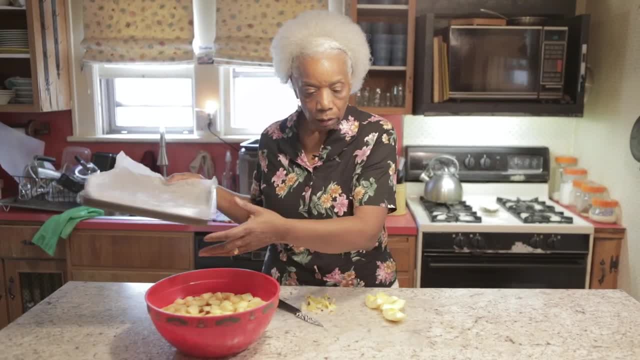 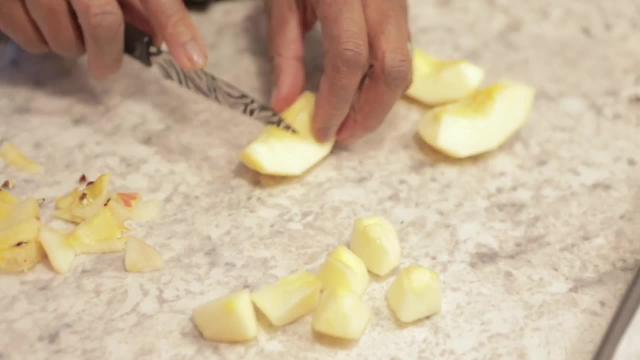 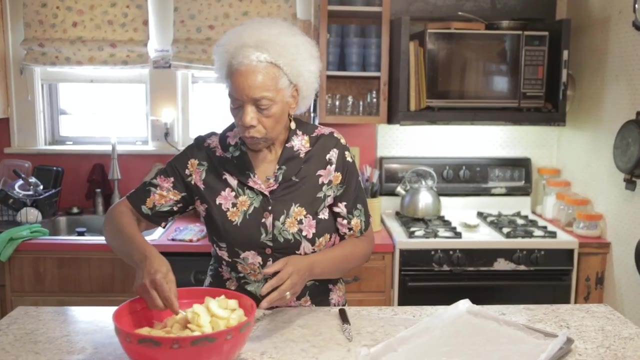 it up really well, and then get a parchment lined cookie sheet, cut it in chunks like that, which I like, but you can also slice Like that- stir it up, stir up your apples and your lemon water, Okay, And then really, 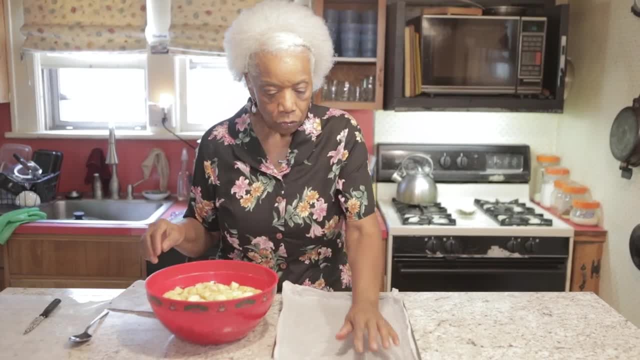 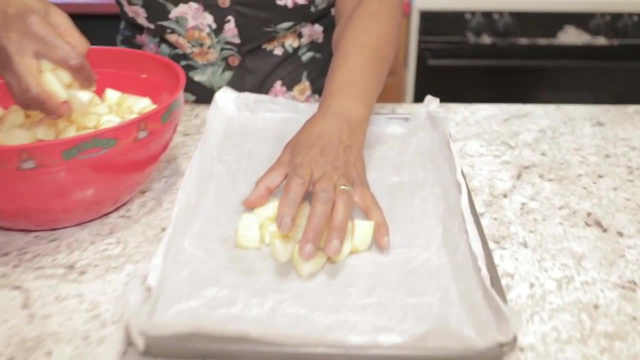 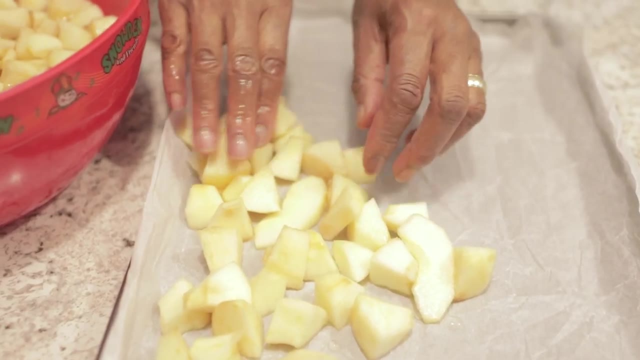 that's all you have to do. You're done, Got your cookie sheet. You just take your hand. You don't like everything. I don't know things. you cook, You freeze. What you want to do is make sure they're in like a single, single line. 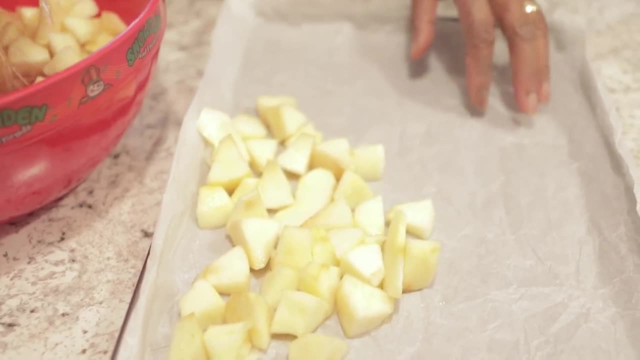 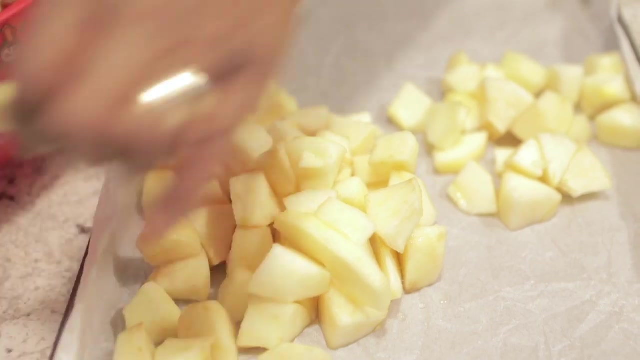 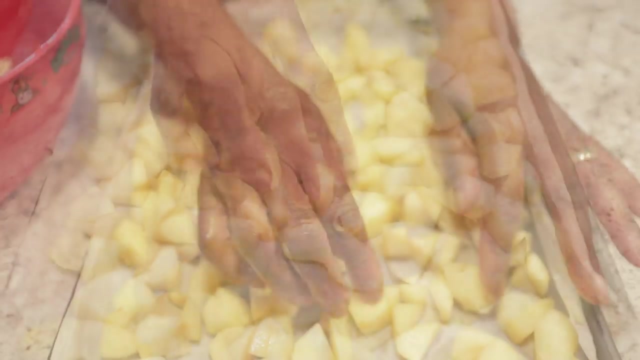 Okay, Can be bunched close together, but you don't want to have a mound, You don't want it like that. Okay, You don't want that, You want it just laying out. They are put on a parchment lined pan. I'm using a cookie sheet You could use. 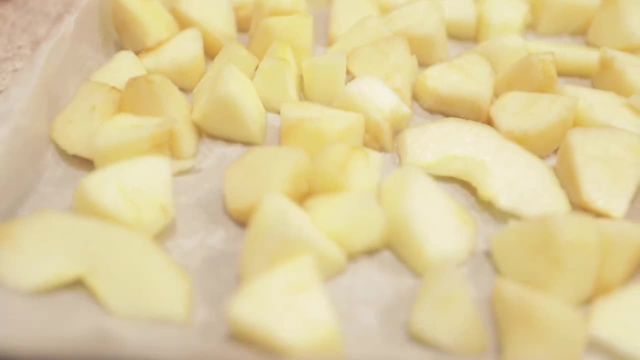 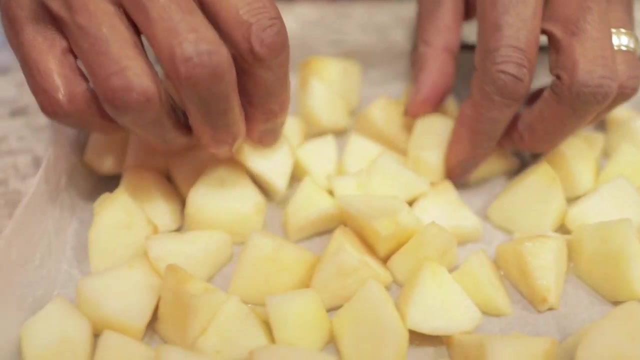 and you know, if you only have a few, you could use an eight by 10,, eight by eight or a nine by nine Square pan. The reason I do this is so that you could take them and throw them in a bag if you. 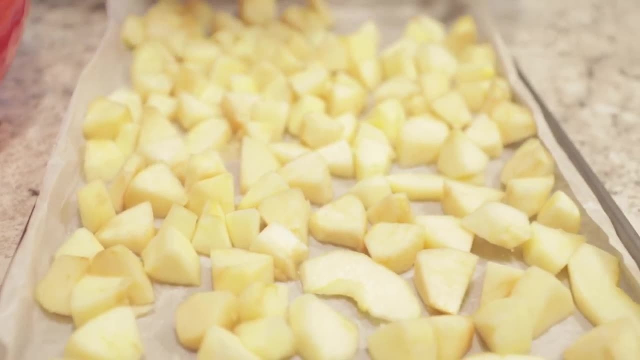 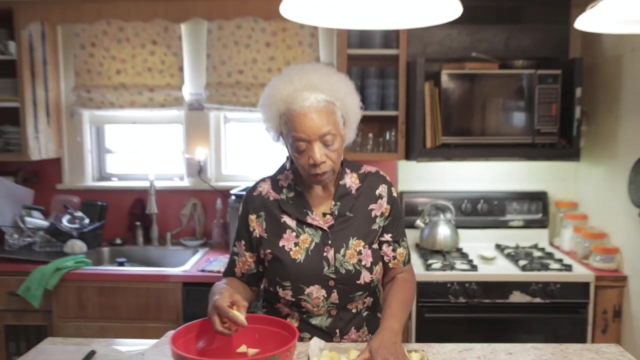 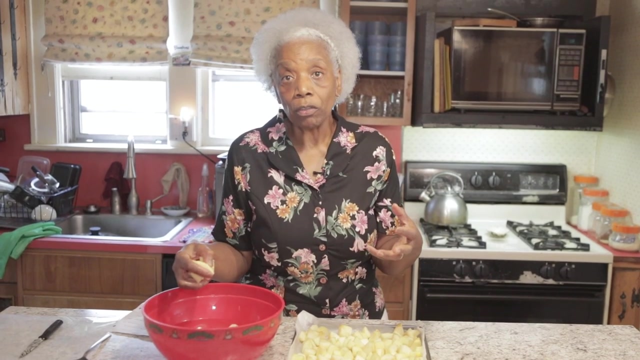 wanted to, But what ends up happening is because they are, the apples are mound on top of one another and they're not laying out flat. You'll get a mound of apples all bunched together in a baggy, in a some kind of a freezer bag. So if you lay them out like that, they'll be individual. So 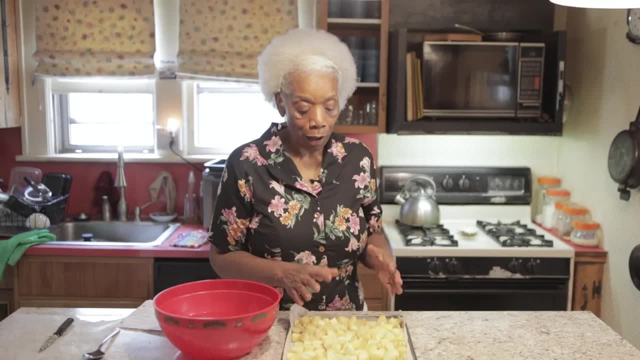 you could take out six or seven. Won't be able to do that. If you put it in a bag, I'll put these in the in the freezer and then I'll bring them out tomorrow. I'm just going to freeze them overnight, You don't have to worry about. 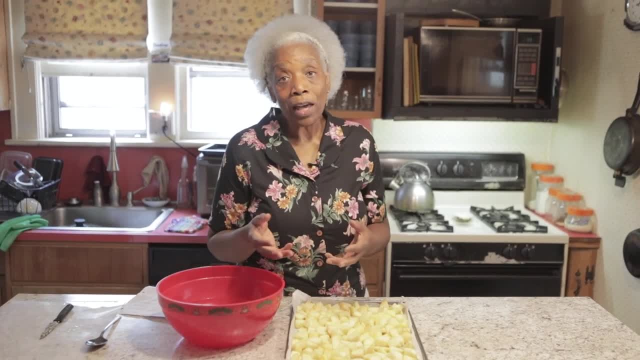 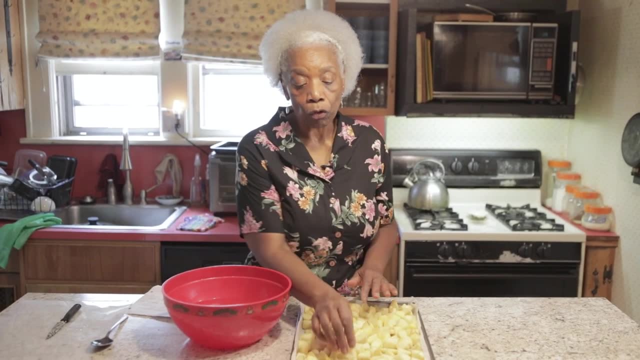 running back and forth a few hours here and there. You can do a free out a few hours if you want to let it be at least four or five, but if you do them overnight that's perfectly okay too. So they're nice and frozen, And I'll just show you what we'll do after we bring them out of the. 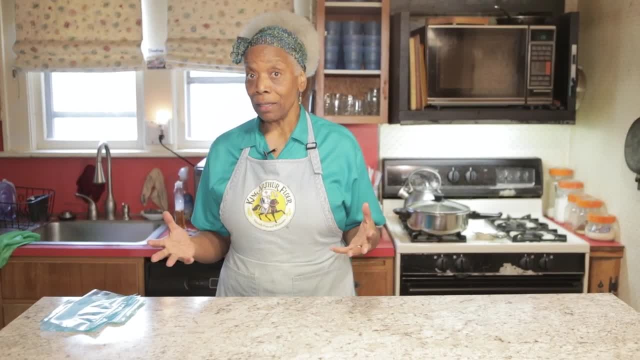 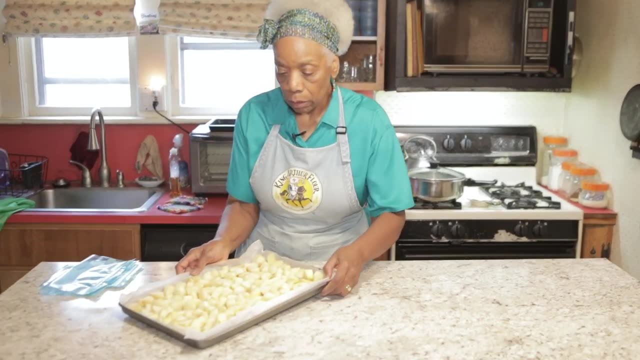 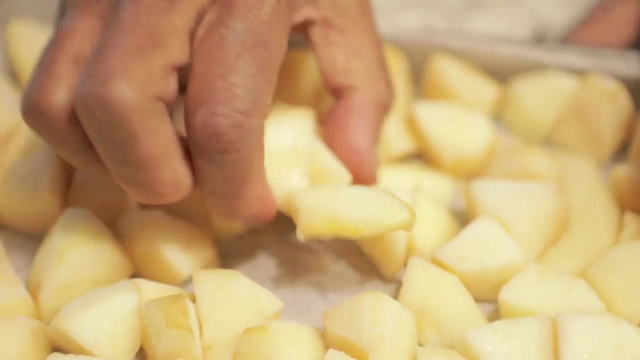 freezer. Okay, So it's the next day and I've frozen all the apples On the cookie sheet And this is what they look like. You see, there's a little bit of frost on each one. Thought I could easily- there we go And they're separate- See that They'll break.